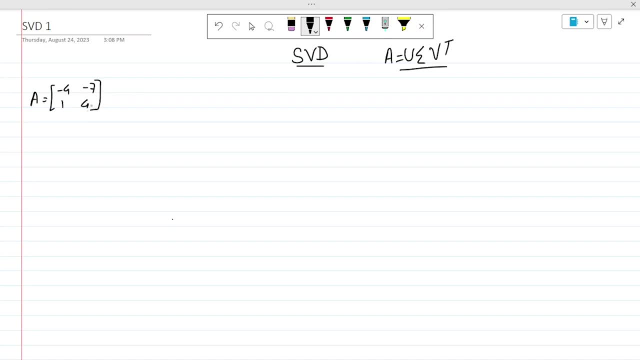 So it is a very small 2 by 2 matrix. So the first step to do any Singular Value Decomposition is to find out the transpose of the original matrix. So A transpose will be always minus 4,, minus 7, it is just like row and column you are just reversing. 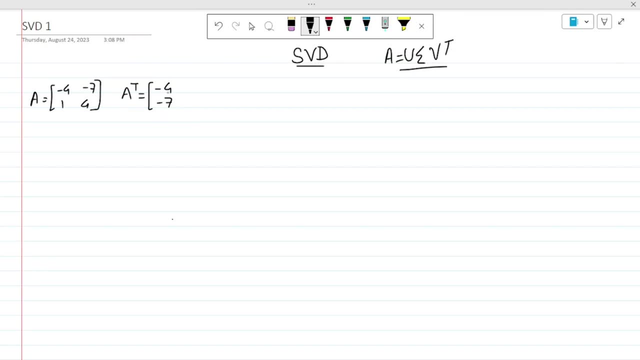 Minus 4, minus 7 was in row. now it is in column. Similarly, 1 and 4 was in row, wise. now it also should be in column wise. So this is our A A transpose, first matrix. So now in the step 1 we have to multiply A A transpose. 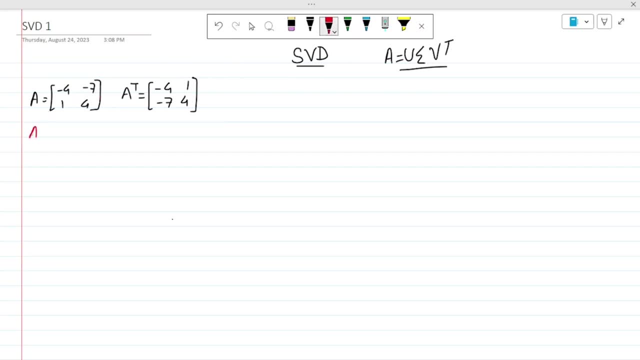 So now in the step 1 we have to multiply A A transpose. So now in the step 1 we have to multiply A A transpose. So we have A matrix and A transpose. matrix multiplication will be minus 4, minus 7 is our A matrix 1, 4.. 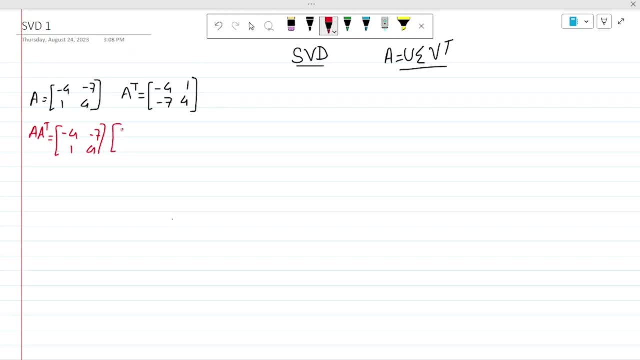 So this is our A matrix and A transpose matrix will be minus 4, minus 7 and 1 and 4.. So if you multiply- this is a simple matrix multiplication- it will follow like that. So minus 4 into minus 4 will be 16.. 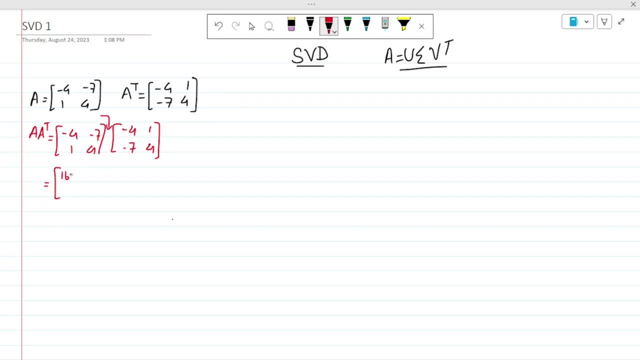 So if you multiply- this is a simple matrix multiplication- it will follow like that. So if you multiply, this is a simple matrix multiplication- it will follow like that. So this is our first value, So this is our first value. Then second value will be minus 4 into 1, will be minus 4, and minus 7 into 4 will be minus 28.. 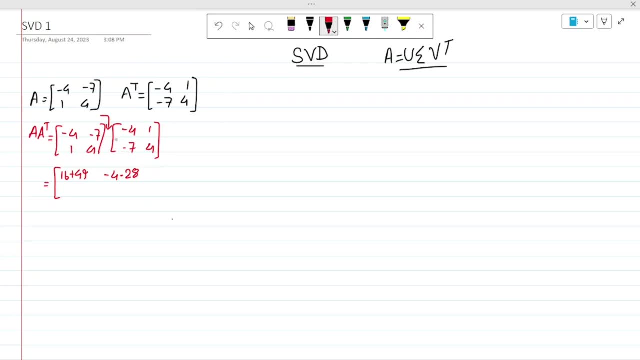 So this is second value. Third value is: 1 into minus 4 is again minus 4, and 4 into minus 7 will be minus 28.. And last value will be: 1 into 1 is 1.. 1 plus 4 into 4 is 16. so this is the matrix multiplication. so what we get at the end is: 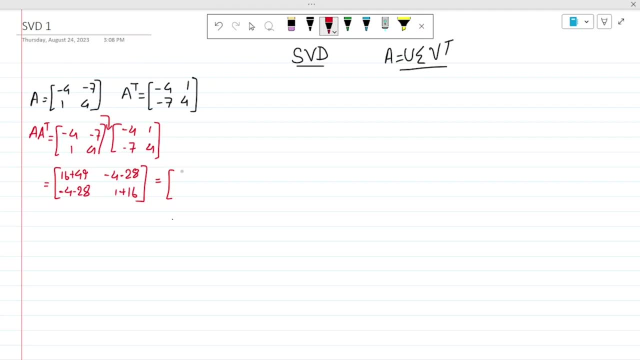 49 plus 16 is 65. then we have minus 4 minus 28 is minus 32. similarly, minus 4 minus 28 is here also minus 32. and then 16 into 1 is 16 plus 1 is 17. so this is the matrix. we got it after. 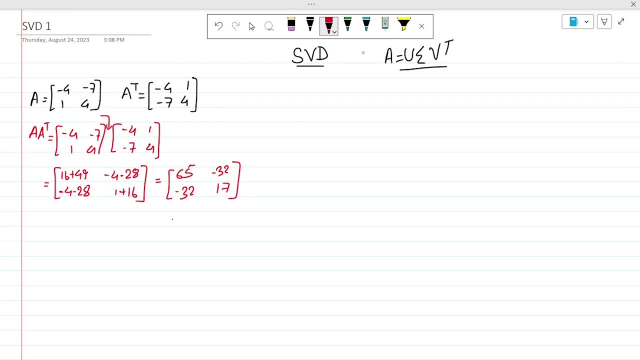 multiplying a, a transpose. so now the third step is: we have to find it out, eigenvalues of this matrix. so how to find it out, eigenvalues. so, eigenvalues, finding out. we have the equation for that. so equation is a, a transpose minus lambda i. so this determinant, determinant of 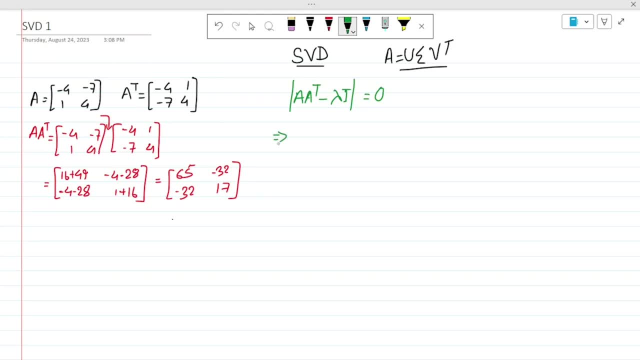 this matrix must be equal to 0. so that's how we find it out. eigenvalues. so a a transpose already we might like. so this is the final value. so simply just plug in the value 65 and we have minus 32, similarly minus 32 and 17. so this is our a? a transpose now minus. 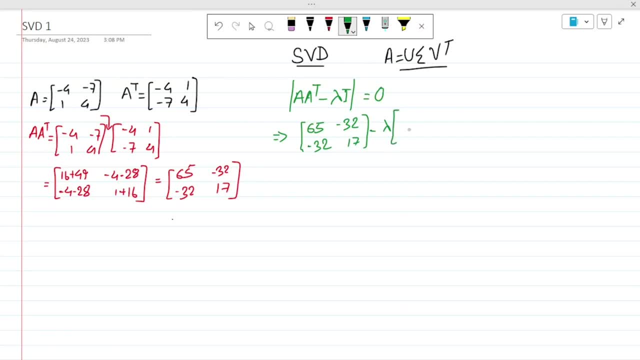 lambda I. so I is identity matrix. identity matrix is nothing but 1, 0, 0, 1. so now, if I do, this is simply matrix subtraction. so you have 65 minus. so lambda into 1 will be lambda. 65 minus lambda, then 32 minus 32 minus 0. 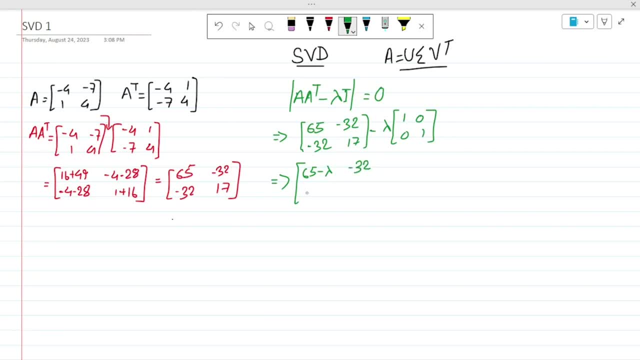 will be minus 32 here again. so here also you have minus 32. and lastly, 17 minus. lambda, 17 minus. so this: a determinant of this matrix must be equal to zero. so then we can find it out: lambda, so determinant. how to calculate determinant is: 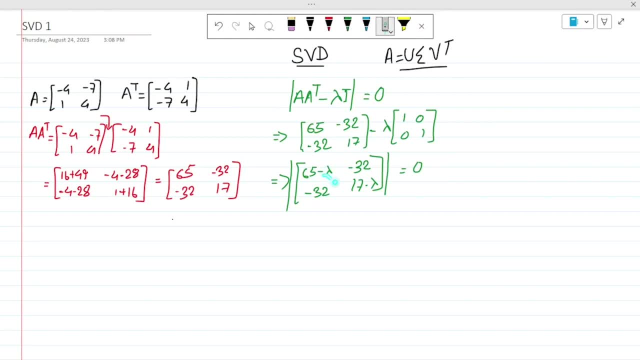 simply just cross multiplication, so determinant will multiply this value and this value, minus multiply this value and this value. so let's do it quickly. so we have 65 minus lambda. this multiplied by 17 minus lambda, so minus 17 minus lambda. minus minus 32 into minus 32. so minus 32 into minus 32. so this must be equal to zero. so now, if we 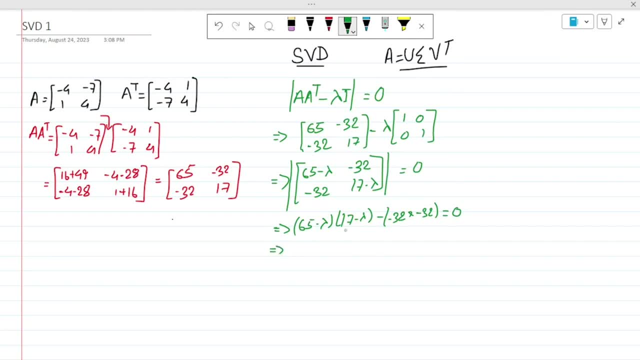 simplify this equation. what do we get? 65 into 17 is 1 1 0 5. so 1 1 0 5. then 65 into minus lambda will be minus 65 lambda. then you have minus lambda into 17 will be minus 17 lambda and then minus lambda, minus. 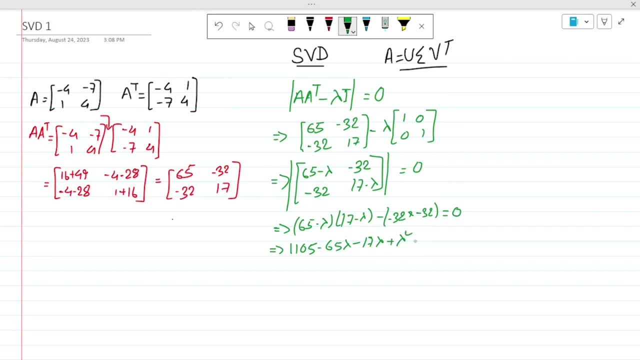 lambda plus lambda square, then here you have: minus 32 into 32 will be 1 0 2, 4. 1 0 2 4, this equal to 0. so now, if we simplify this equation, we get lambda square minus 65 and 17 will be 82. lambda plus 1 1 0 5 minus 1 0 2, 4 will be 81. this must. 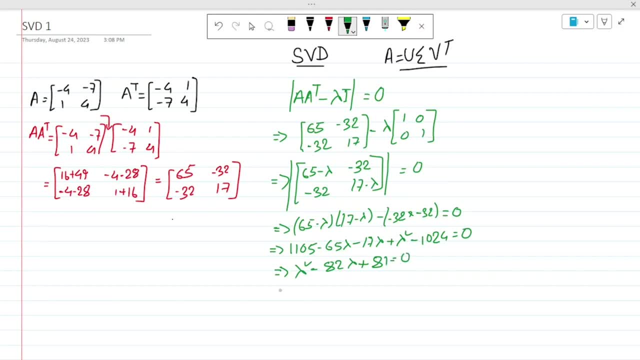 be equal to 0. so next we can easily decompose this equation: lambda square minus 81, lambda minus lambda. so 82 lambda can be decomposed into 81 lambda, and 1 lambda plus 81 must be equal to 0. so now again we we try to take the lambda common here. so 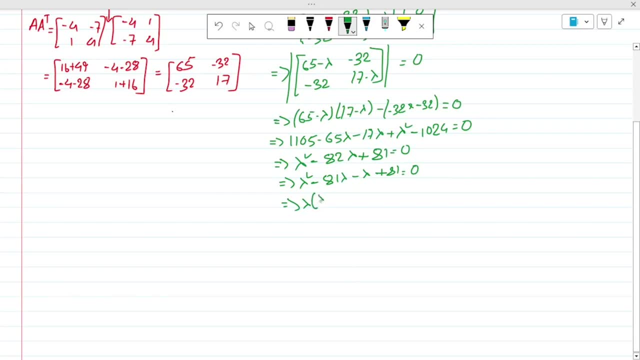 what we get is lambda minus 81. so lambda minus 81 minus 1- common again. so here also we have lambda minus 81 equal 20. so from here again in, what we get is нам エ, iat ist 是, and also lambda minus 1 equal to 0. so from this equation we can easily find it out what is the. 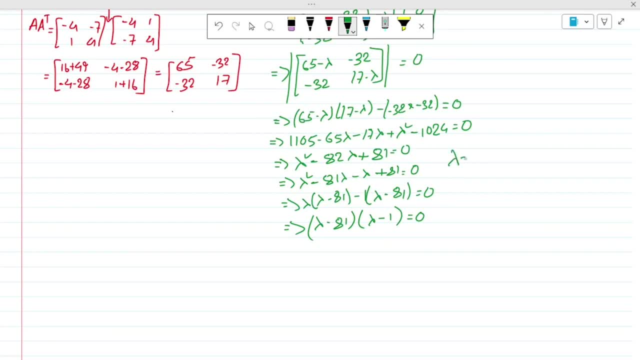 value of lambda. so lambda value will be: so lambda value will be 81 and 1, so two lambda values. we got it after solving this equation, and this equation is called the. these two values are called eigenvalues of the matrix. so now from here we have to compute these three matrices. 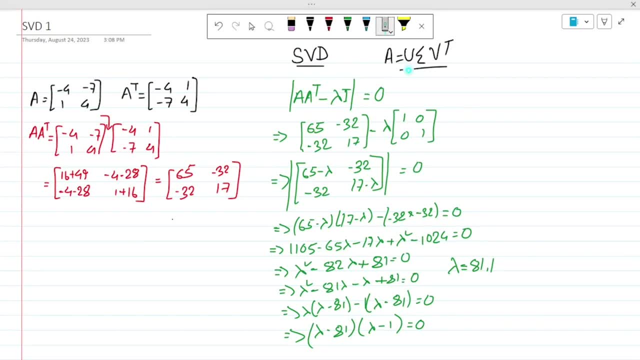 right. so u, v and so these three matrices- we have to find it out- u, sigma and vt. so, as we already find it out, sigma value is 81, lambda value is 81 and 1. that means we got this middle matrix. so now how to rewrite the middle matrix. so middle matrix sigma will be equal to first value. we got it 81. 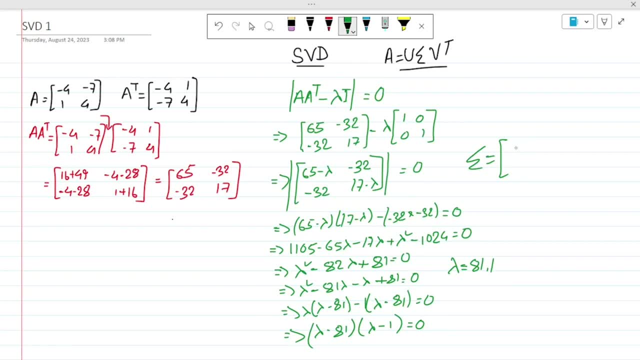 so always, first value should be higher. eigenvalue should be written at the top position, so it will be square root of 81 and then 0 and here 0 and here. second value is 1, so square root of 1. we have to write. so this is our sigma. 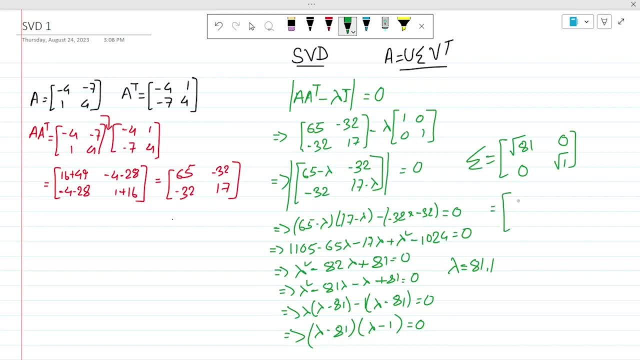 matrix, which is the diagonal matrix. so if you simplify, square root of 81 is 9 0, 0 and square root of 1 is 1, so this is our first matrix, which is sigma matrix. now, and this value is this: values are also called eigenvalues. so now the next step, step. so in the first step we have just multiplied. 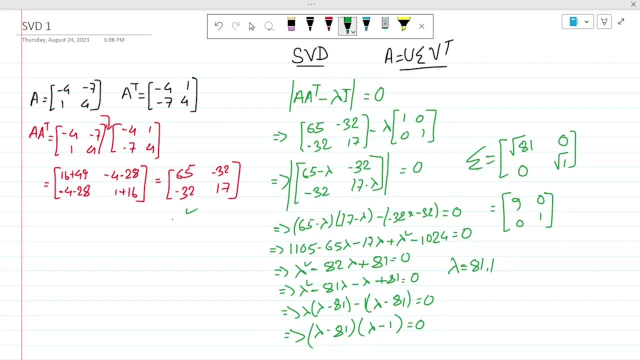 these two value. in the second step, we calculated the eigenvalues and we got the second matrix, which is sigma matrix. now, in the third step, we have to find it out eigenvectors based on these eigenvalues. so let's find it out eigenvectors of this equation. okay, so now here we. 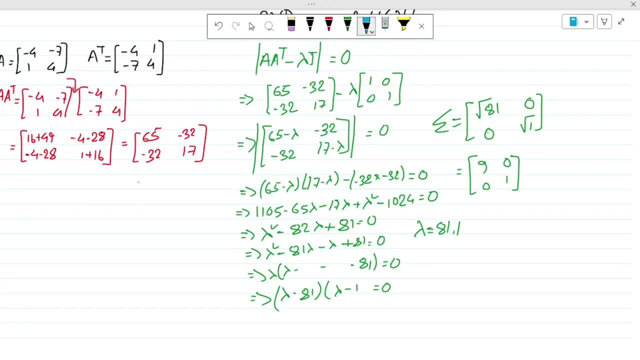 have two eigenvalues, one is 81, another is 1, so let's find it out eigenvectors for each of these eigenvalues. so first we will find it out eigenvector for 81 and then we will find out eigenvector for 1. so let's get started. so first, 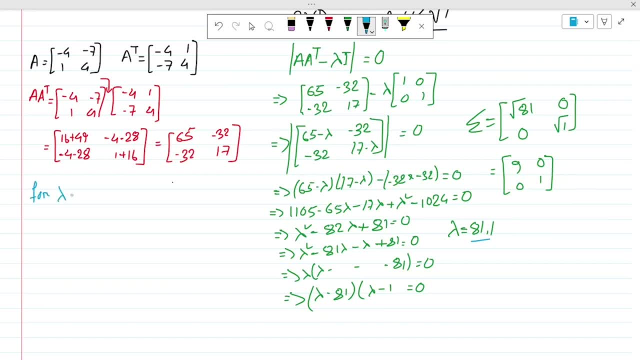 for lambda equal to 81, what will be the eigenvectors? so how to do it? the equation is same which we have used earlier, so it is a, a transpose, a, a transpose minus lambda i. earlier we have used here we have used a transpose, lambda i. so here now lambda value, we will put it 81 and i is basically. 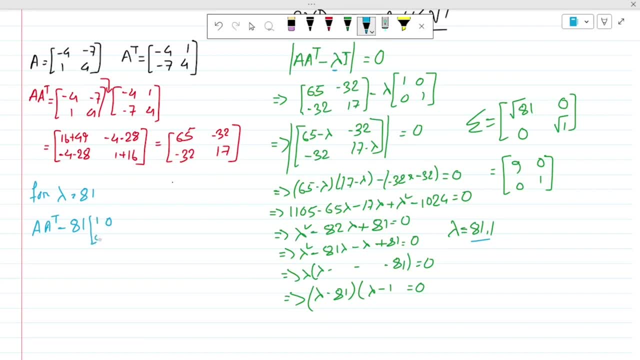 our identity matrix, which is 1, 0, 0, 1. so this dimensional matrix will be multiplied, multiplied by, so this vector into V once, v11, v2 one, so this two are two eigenvectors for 81, and this must be equal to 0, 0. so now, from here let's. 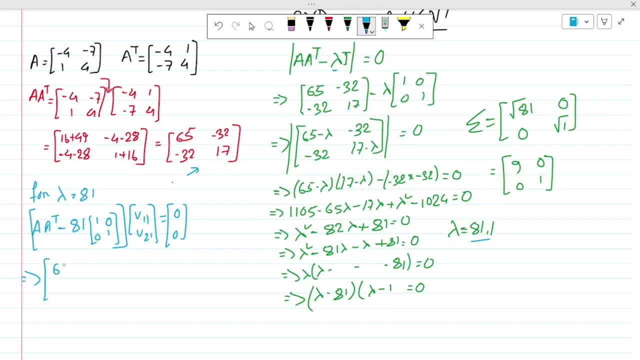 substitute the values. so first is a a transpose, a transpose already we have calculated the same value will give me at 65, and then we have minus 32, and minus 32 minus, we have this 81i. So 81i means 81 into 1 is 81.. 81 into 0 is 0.. 81 into 0 is 0.. 81 into 1. 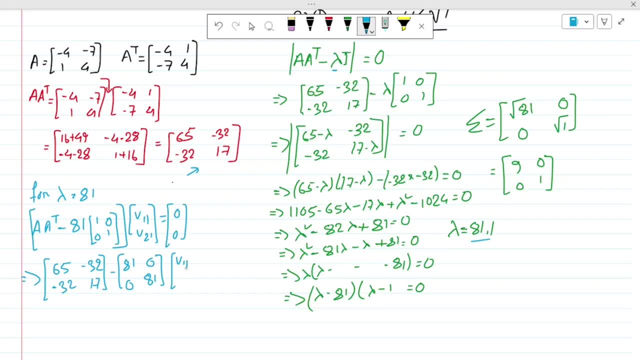 is 81.. So this into v11 and v21.. So our objective is to find it out: v11 and v21 for now. So, and here it is 0, 0.. So now let's find it out these two values. This is simply a metric subtraction. 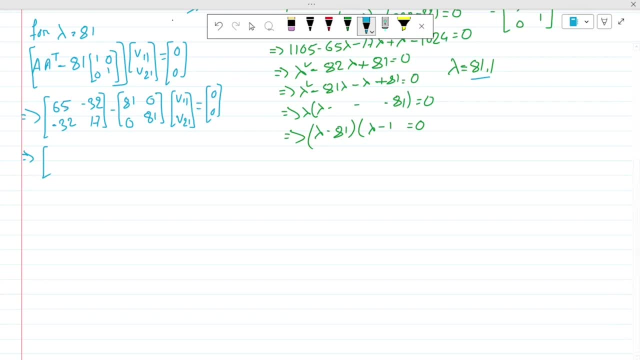 So how will you do metric subtraction? Simple, So 65 minus 81.. 65 minus 81 is minus 16.. Then you have 32 minus 0.. Minus 32 minus 0 is minus 32.. Similarly, minus 32 minus 0 will be. 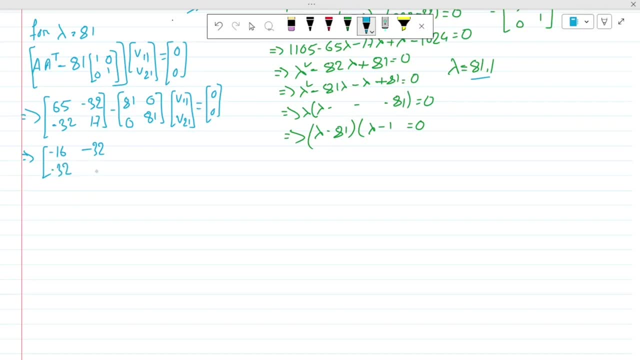 again minus 32.. And 17 minus 81 will be minus 64.. So this is our first metric. Second metric is same v11 and v21, and this equal to 0, 0.. So now, from here, what we get it is: we simplify Now, if you see, all elements in this matrix has 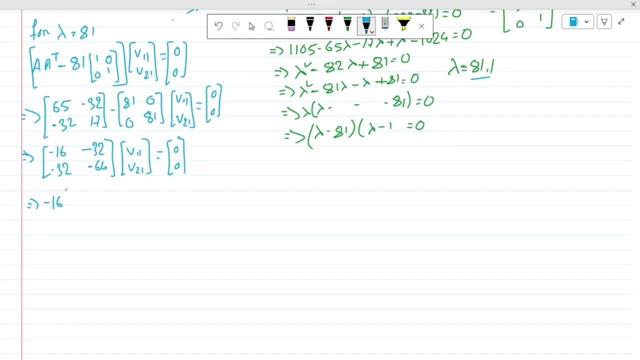 16 common right, So we can take minus 16 from out everywhere. So minus 16, then you will have 1 here. So 1 into minus 16 is basically minus 16.. Similarly, from here you will get 2.. So 2 into. 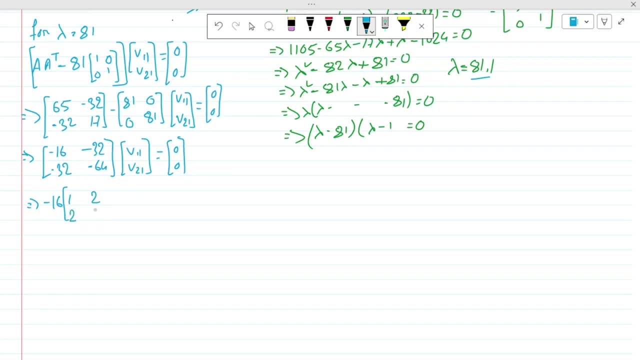 minus 16 is minus 32.. Similarly, here also 2. We just simplified this and this will be 4.. So 4 from all the 4 elements, And then you have v11 and v21. So these two values, and this must be equal. 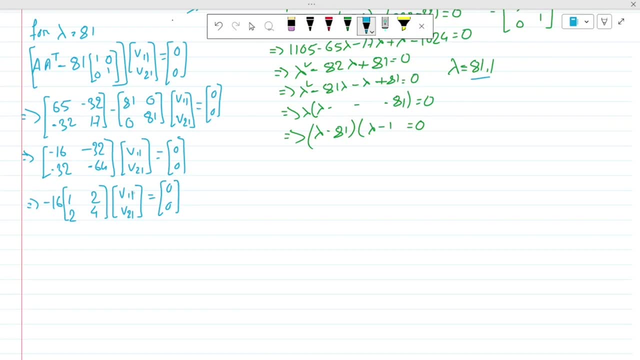 to 0, 0.. So we are finding out v11.. So, as we can see, this side is 16 and this side is 0. So we can simply remove those 16 from the equation. So finally, we have 1, 2,, 2, 4 equation. I mean. 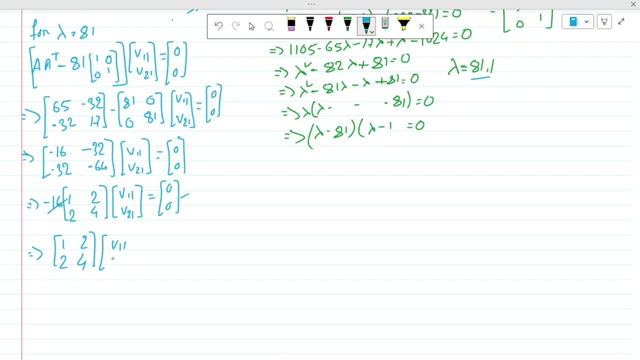 metrics and also this side. you have v11 and v21. This equal to 0, 0.. So now we have to find it out v11 and v21.. So how to do it? It is again simply matrix multiplication. So matrix multiplication will be v11.. So 1 into v11 plus 2 into v21, and this 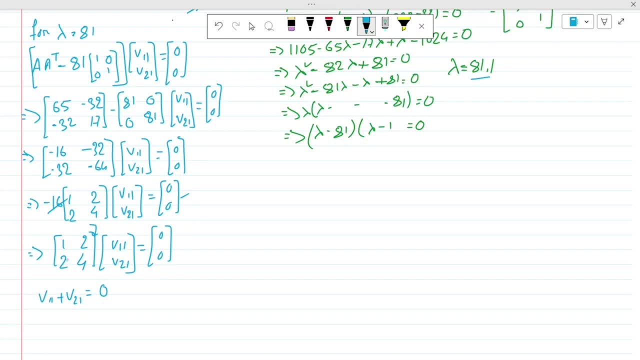 equal to first row is 0. Similarly, 2 into v11.. From second row we get it 2 into v11 plus 4 into v21.. So 4 into v21. Let me erase this part. Yeah, So the next part will be 4 into v21, equal to 0. So now we have to find it out: v11 and v21 from this expression. So here, also from, if you see, from second expression, you can take 2 common Right, then you have v11 plus 2v21, equal to 0.. Because what I have done, I did 2 common Right. 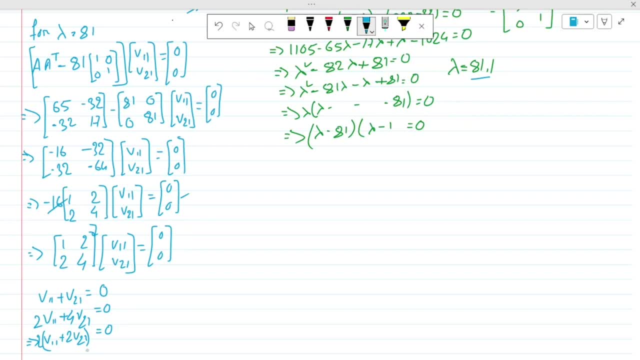 from entire expression, Then again 2, 2 will get cancelled out. So finally we have: from second expression is v11 plus 2v21 equal to 0. And from first expression also, if you see: 1 into v11 plus 2 into v21. So here we missed: 2 into v21 is equal to 0. So now if you see this expression and this: 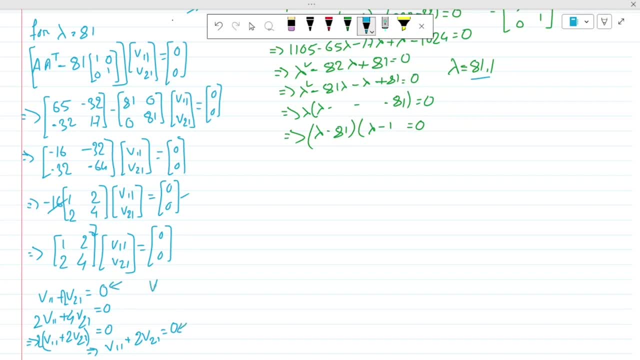 expression. both expressions are equal. That means we can write v11 equal to minus 2v21.. So just if you take v21 this side, then it will be minus 2v1.. So this is our expression, eigenvalue expression. So now, if you consider v21 value as a 1, then what is the v11?? So let's. 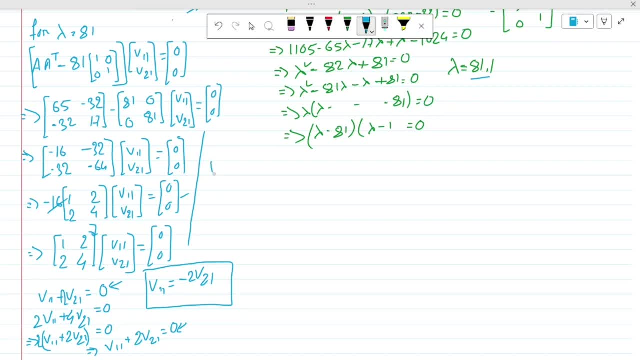 assume, let's assume, v21 equal to 1.. Then what will be the value of v11?? So v11 will be, simply, if you put it, 1, v21 below is 1, then v11 will be minus 2.. So minus 2.. So. 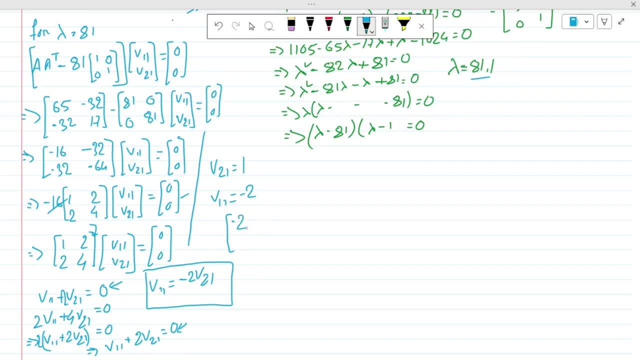 our first vector we got. it is: v11 is minus 2 and 1 will be. this is our first eigenvector. So from 81 we got it right. So if you consider lambda is equal to 81, then our eigenvector is: 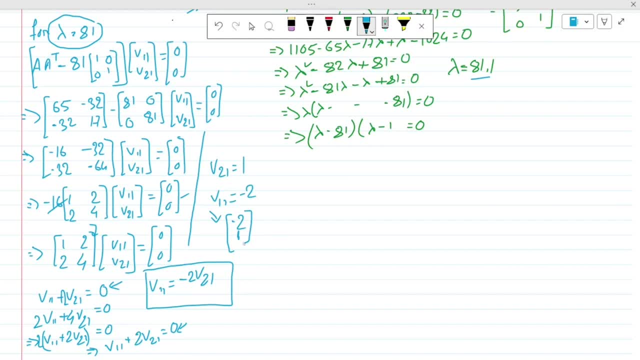 this one minus 2 and 1.. So minus 2 and 1 is the first eigenvector. So now we have to simplify this expression. This is not a unit length. We have to make it as a unit length. So how will you do it? So we have to. 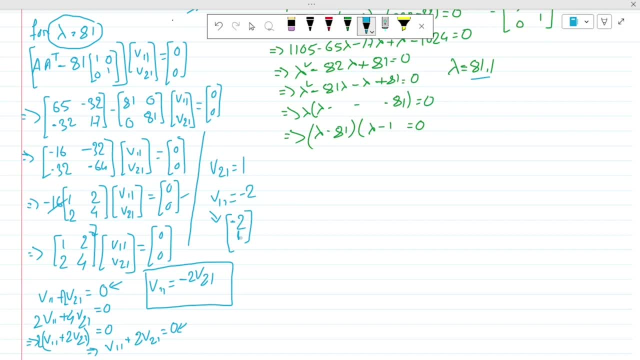 divide this entire vector into a. it's the length. So what will be the length of the vector? Length of the vector. for example, you have two matrix, a triangle, right. So if this side is a and this side is b, then what is the length of this, this portion? So if this portion is c, then c is equal. 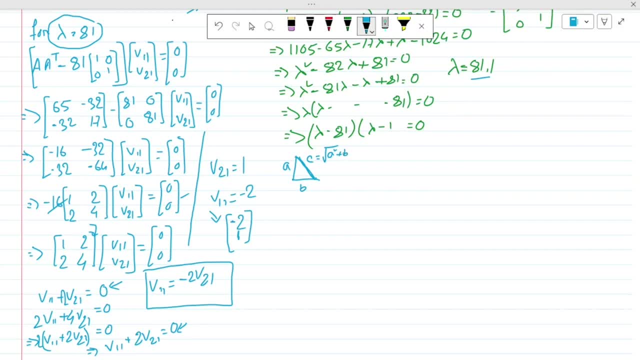 to square root of a square plus b square right. So this is the length of this vector, right. So same thing. So here also, what will be the length of this vector? So length of v11 and v21 vector. 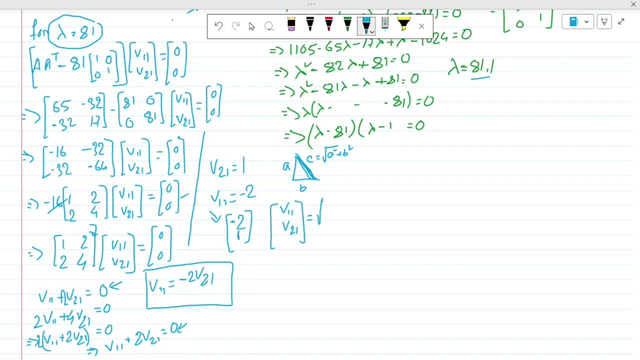 So length of this vector will be equal to square root of root. minus 2 square means a square plus second value is 1, 1 square. So if you solve it you will have root over 5,. right 2 square is 4. 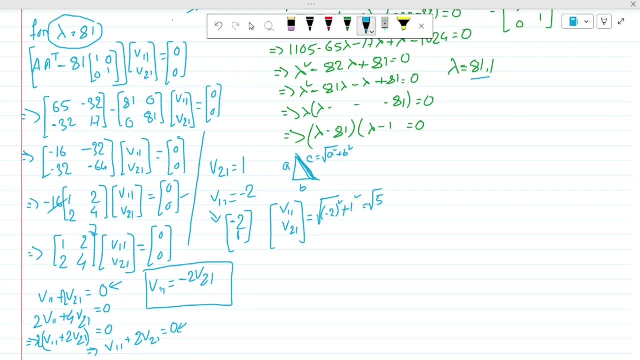 plus 1 is 5.. So root over 5 is the length of the vector. So now, whatever, we got it eigenvalue, So from here we have to divide it by length of the vector. So the eigenvector. so let's formally 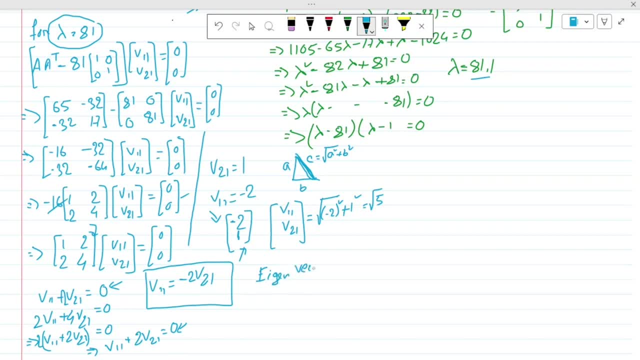 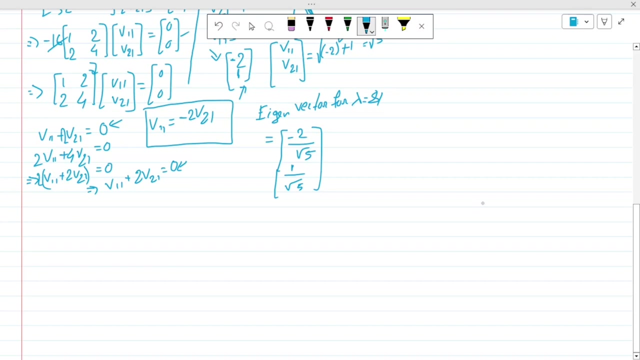 write it: eigenvector for lambda is equal to 81, equal to what we get. it is minus 2 divided by root 5, and then you have 1 divided by root 5.. So this is the eigenvector for the, for the lambda value of 81. So similarly, we can find it out: 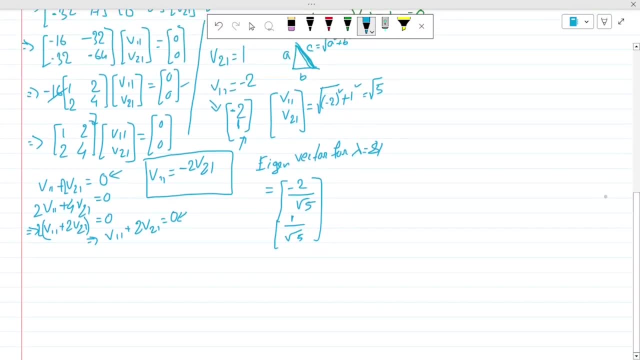 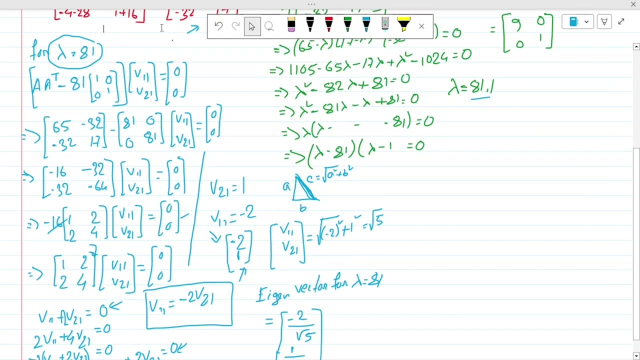 eigenvector for lambda is equal to 1.. So this eigenvector, what we have got it we considered lambda is equal to 81. So now let's this: this is lambda is equal to 81. So now let's do same. 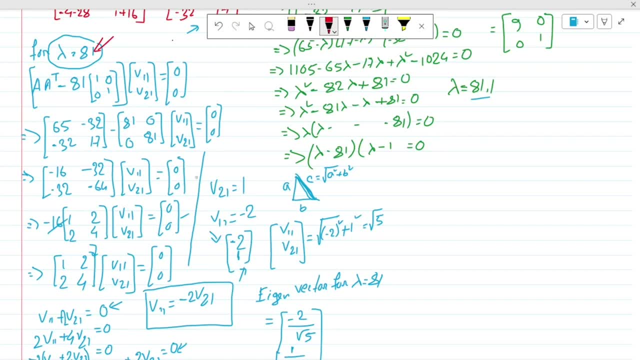 process the same blue color color. whatever I have done same thing. let's do it with. lambda is equal to 1, because we got lambda value is 2, 2 values. So this is the eigenvector for lambda is. 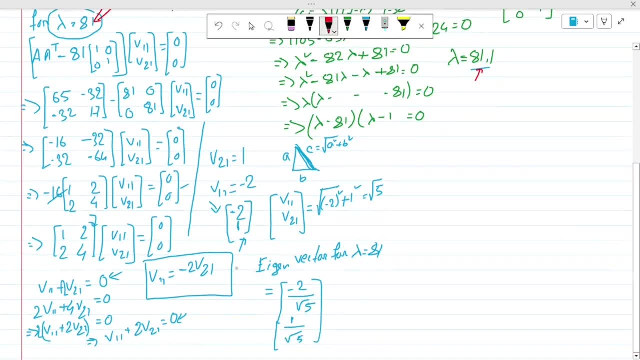 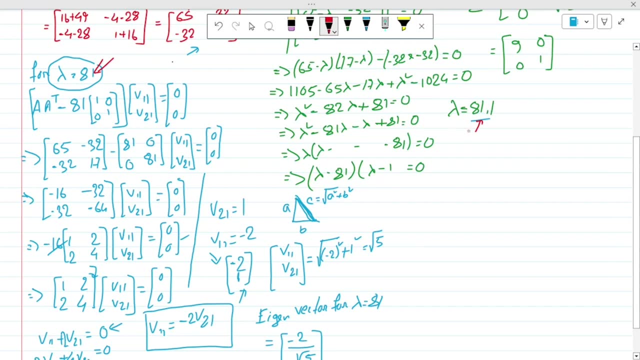 2, 2 values. One is 81,, another is 1.. So for 81, we got. this is the final expression. Similarly, same thing, we'll repeat it- for lambda is equal to 1.. So let's do it. So now. 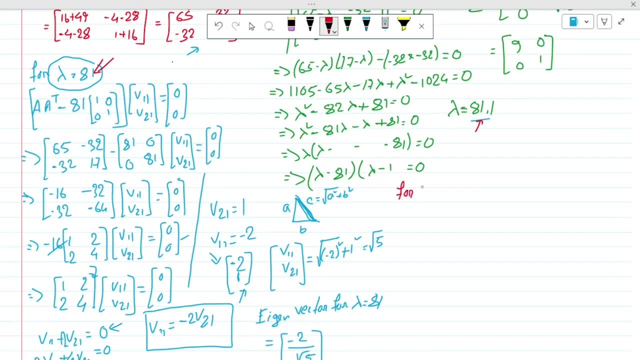 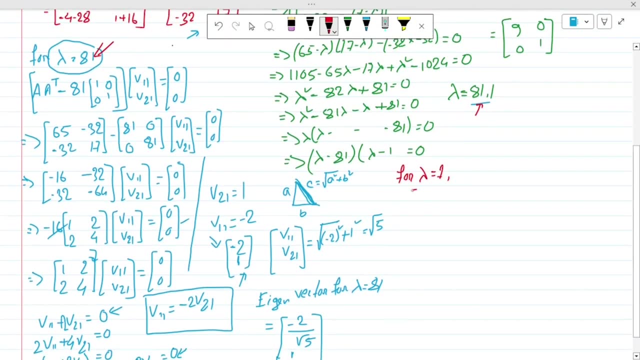 for lambda is equal to 1,. what is the value? Let's do it So: same equation, same expression here. what we have used, the same expression, same expression. we'll use it now also, So it will be same thing. 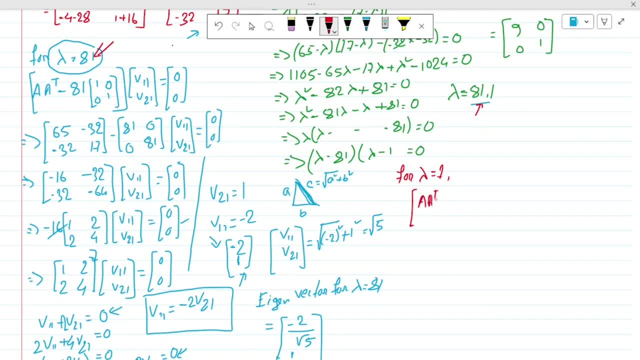 So this is elementary what happened here. this is 1 and this is 1.. So instead of 1, you will get small, neither small nor real- of 1.. So this 0 above something is 1.. What was that? 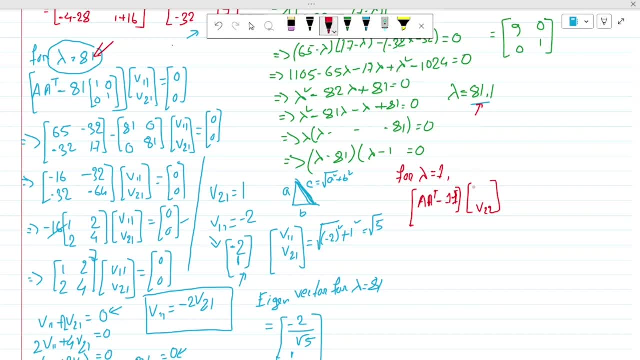 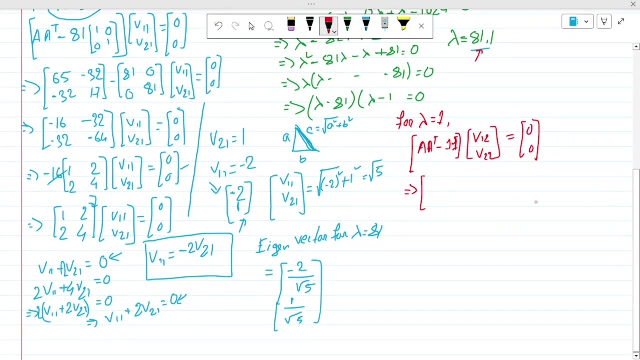 What was this? so it will be v12 and v22, equal to again 0 by 0, 0 matrix. same process will be repeating now. so aa transpose. already we have calculated which is 65 into 65, 32, 65 minus 32 minus 32, and here it is 17. so this minus 1i, i means again identity matrix, which is 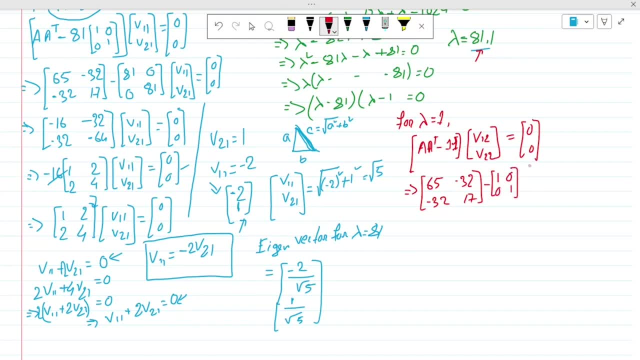 1 0, 0, 1. so this again: v 1, 2, v 2, 2 will be there: v 1, 2, v 2, 2. this equal to 0 by 0, 0 matrix. so now, if you do matrix subtraction, what you will get it is 65 minus 1, will be again 64 minus 32 minus 0. 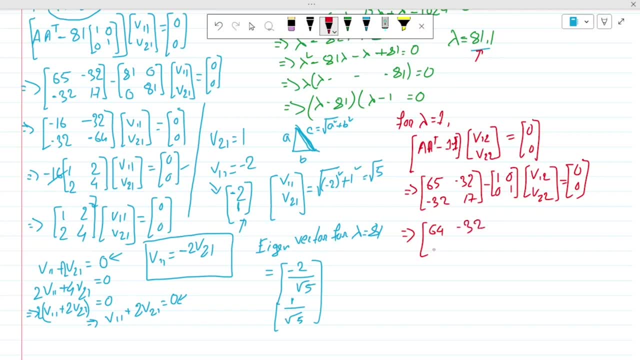 will be minus 32. so minus 32 minus 0 will be again minus 32, and 17 minus 1 will be 16.. so 16 and this part is same: v 1, 2 and v 2, 2. this equal to 0: 0. 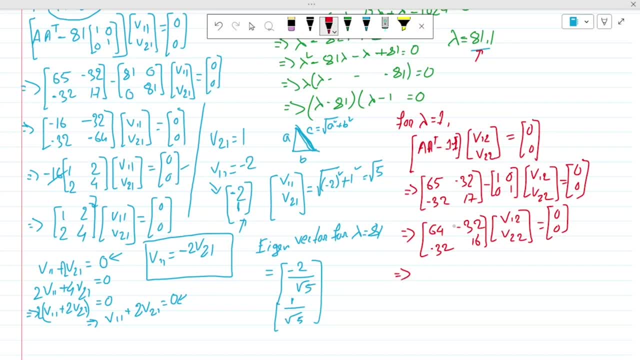 so now again, if you take, if you see, all elements are multiplication of 16. so again, let's take 16 common outside, then you have 4 minus 2 minus 2 and this is 1. so and this side is again same, v 1, 2 and v 2, 2, this equal to 0 by 0. so now, from here, what, what we can do. 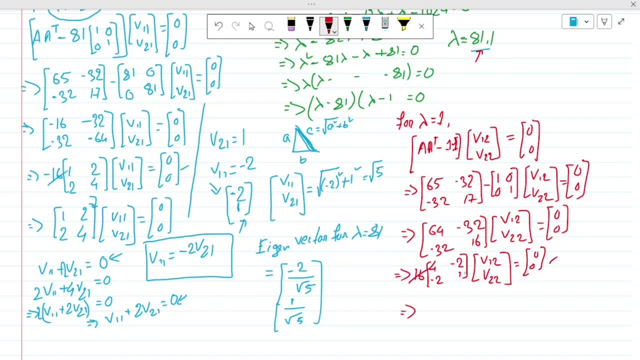 we can again simplify, so this 16 will go with. this side is not there. so this is matrix multiplication from here. what we get it is 2 into same, 4 into v 1, 2 plus minus 2 into v 2, 2, so it will. 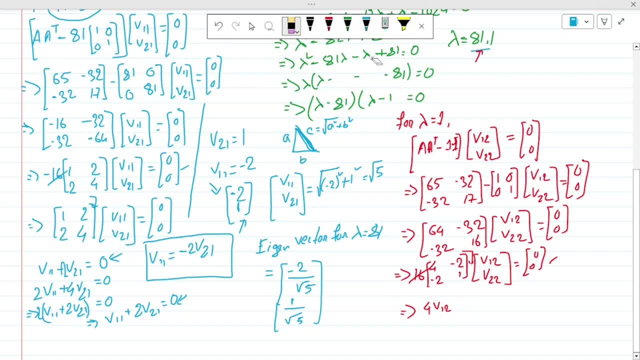 minus 2 into V22.. So it will be minus 2 V22 equal to 0. So, again from second expression, what you get it is minus 2 V12, minus 1 into plus 1 into V22 equal to 0. So now you can. 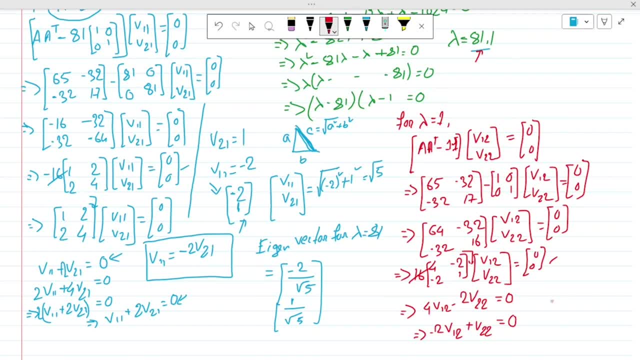 use again both the equations if you see the similar kind, So let's do it here. So you have V12 equal to. from first expression. if you see V12 is equal to 2, V22 by 4.. So this 4 will come this side. So 2 by 4 again it will be 2.. So you will have V12 equal to V22. 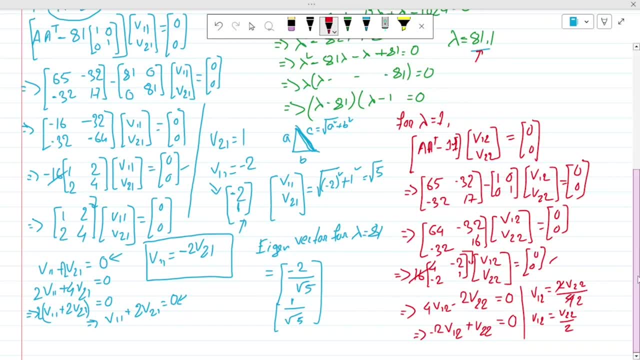 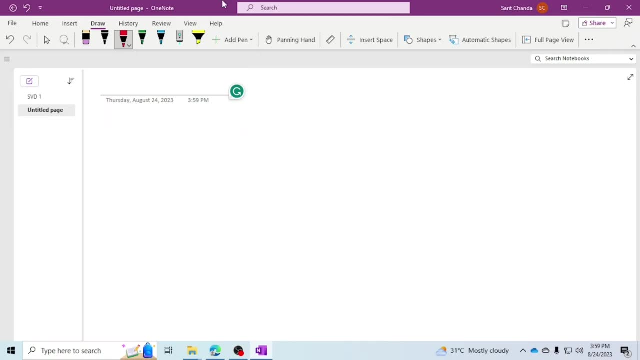 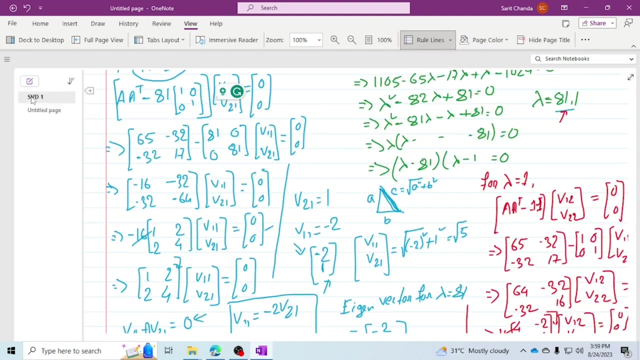 by 2.. So this is the final expression. we got it after solving this one. So again, if you consider V1 equal to, let's do it here, I think. or let's do again. consider one more page: Okay, View ruler. Let me take ruler. Okay, So now here, at the end, what we got it is: this is the final. 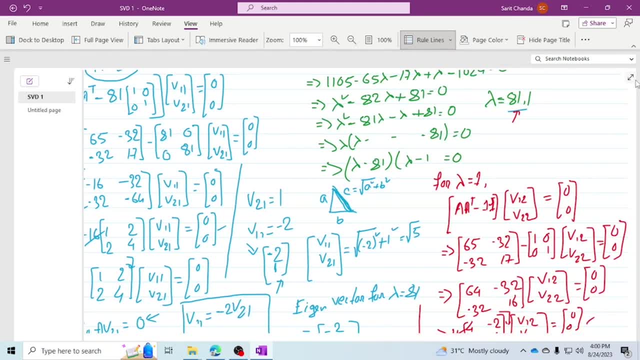 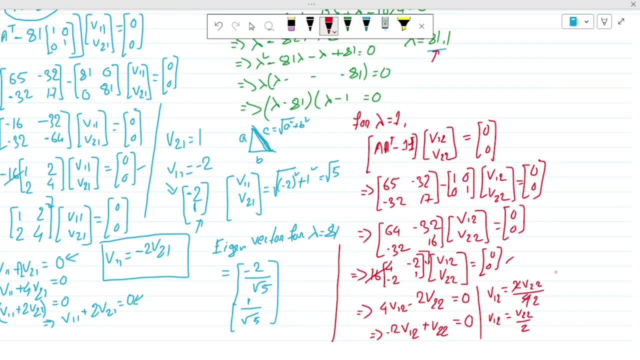 expression. So V12 equal to. So V12 equal to. this is the final expression. Let's do it here. only then this will be easy. So now let's consider V22 equal to 1.. Then what will be the value of V1: 1, 2.. So V12 will. 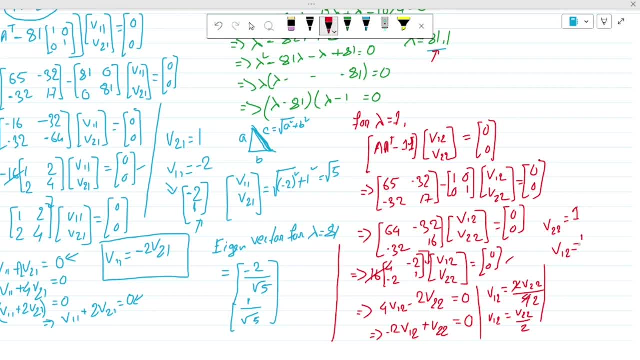 be simply: if you substitute V2 to 1, then it will be 1 by 2.. So ultimately now you have the matrix of 0.5.. Half means 0.5. And half means 0.5. And half means 0.5. And half means. 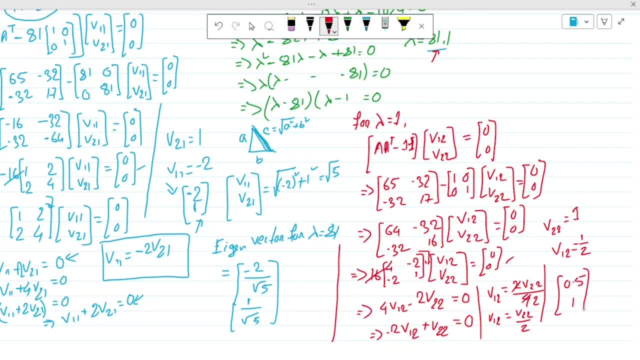 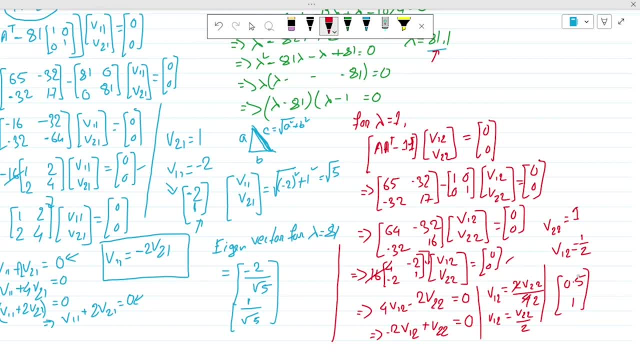 eigenvalue. So again, you have to neutralize, You have to not neutralize, You have to find. divide it by unit vector, So ultimately you have the eigenvector for lambda is equal to 1. equal to it will be 0.5 by square root of 0.5.. 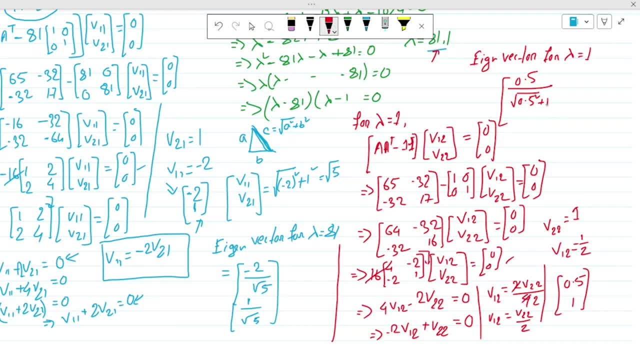 Okay, 0.5 square, same plus 1 square, and it will be 1 by same value. so 0.5 square plus 1 square. so this, if you simplify, you will get the second eigenvector. so these are the two eigenvectors for. 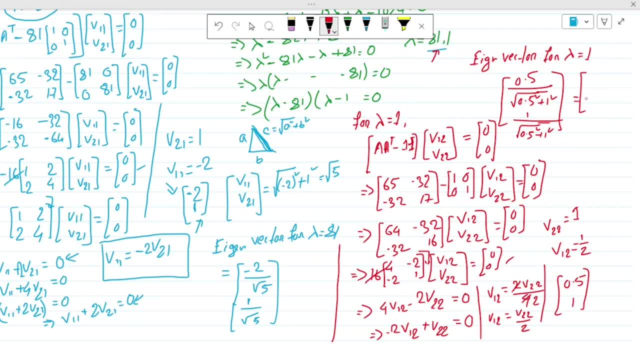 first v1 and v2, 2, so this this comes out to be 0 point 4, 4, 7, and second value is 0 point 8, 9, 4. if you do this up to do these operations, you will get. this is the final value. similarly here also. 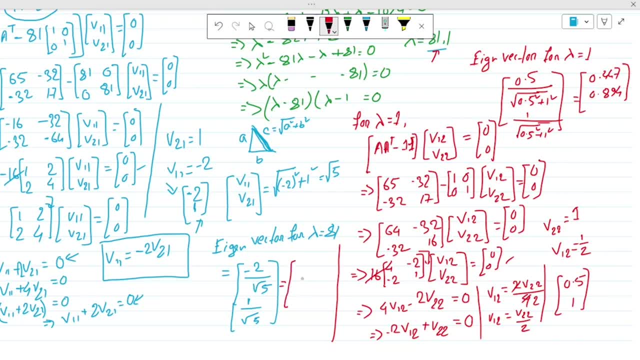 if you do, if you simplify this equation, you you will get minus zero, point 0.89, minus 0.894, and similarly here you will get 0.447. so this, two eigenvectors, eigenvectors, you will get it. this one is for 81 and the second one is for 1, so now we got our. 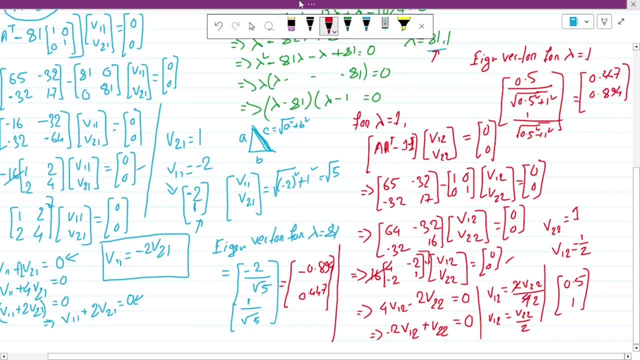 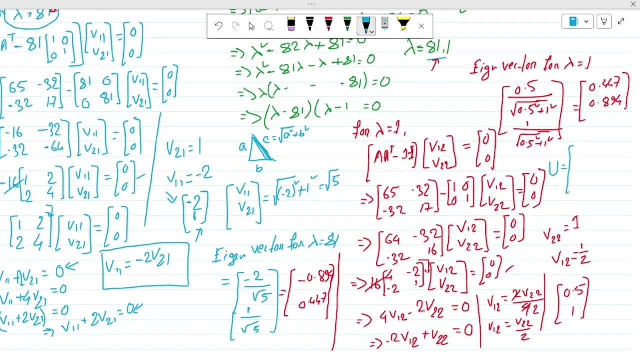 second vector. second vector is our u vector. so let's formally now write u vector, so u vector will be nothing. but so let's do it in the next page. so, okay, i'll write here. only then it will be easy. so u vector will be now. u vector will be now. this one. first eigenvectors for the 81 is 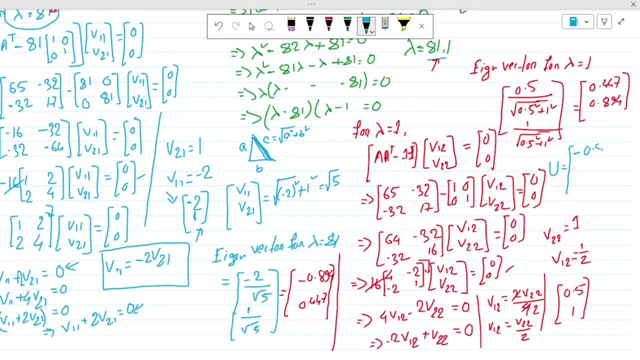 minus 0.894 and 0.447. right, so this is the first vector, so let's do it in the next page. so, okay, i'll write here. only then it will be easy. so u value and second value is the same one. second value is this one. you have to write it here. so 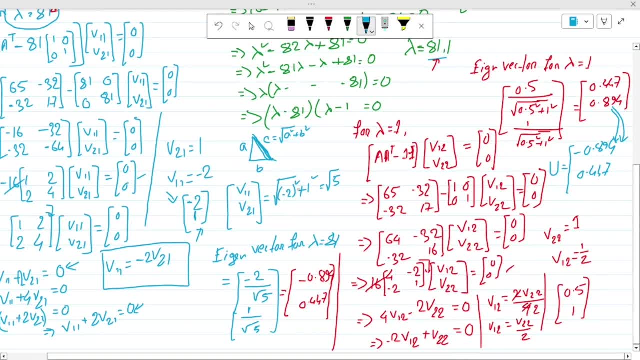 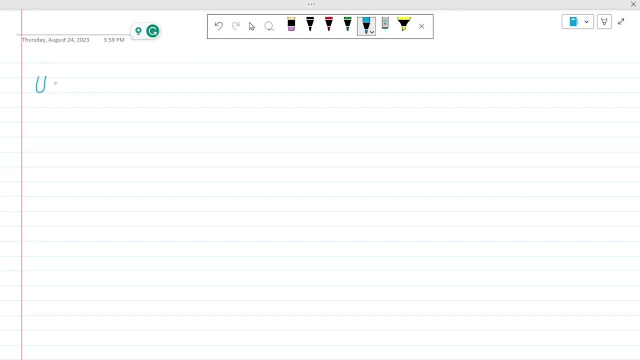 i think there is no space i could not able to write. okay, let me do it in the next page. so finally, our u matrix. let it write it in the second page. u equal to. from first matrix. we got it 0.894 and 0.447. so these two, these values that we got it when lambda was. 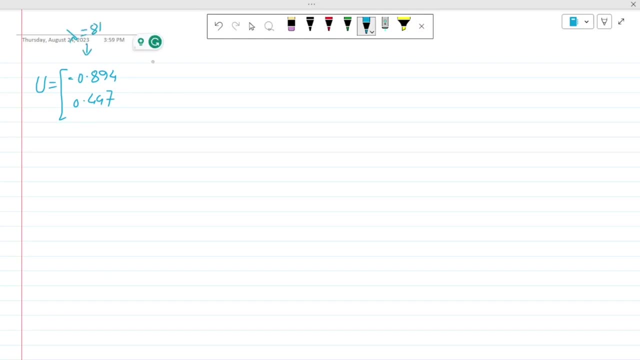 when lambda was 81, we got these two value. and then, when you got lambda is equal to 1, what was the eigenvectors? eigenvectors: we got it minus, not minus. this was plus 0.447. and second value: we got it 0.894. so this first one, we got it. this first one, we got it when the 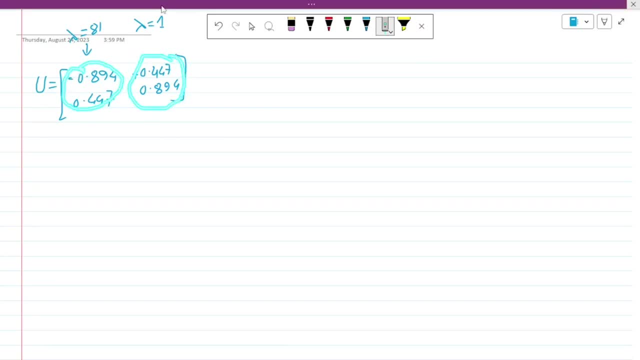 the lambda was 81 and this two value: we got it when the lambda was it lambda was 1, so now let's solve the further one. so we got two matrices: u matrix, also we got it, lambda matrix also we got it. so let me again write u matrix, sigma matrix, what we got it. so 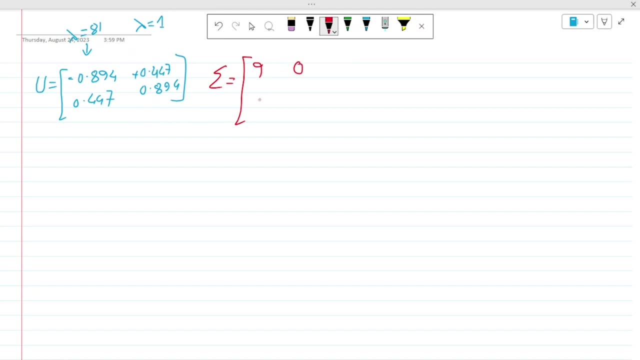 sigma matrix was, you know, 9, 0 and 0, 1. so in the last page we solved so these two matrix. we got it. so what was our objective? if you recall, our objective was a equal to u sigma vt. so these three matrix we have to find it out. so a matrix is given in the equation, u matrix we already 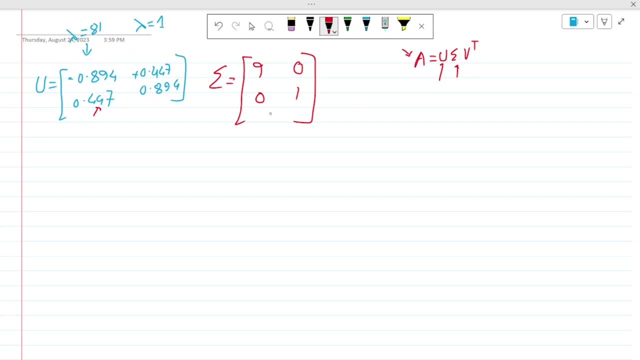 computed. so this is our u matrix and sigma matrix also. we computed, this is our sigma matrix. so now last matrix we have to find it out is the vt, so vt. from this expression you know what will be the v, so vi, so vt. basically, from this you can. so from here, how you can find v so v means you have to. 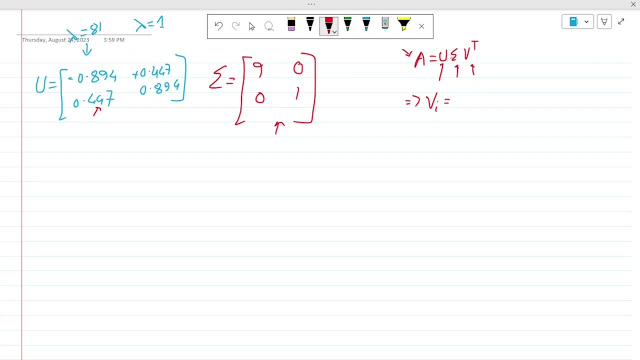 take u this side, u will come. similarly sigma also. 1 by sigma will come. so from this expression you know. so sigma will come this side. so it will be 1 by sigma. you have a transpose, a, transpose u. so from this expression you have to find it out: v matrix, then our problem is solved, so almost. 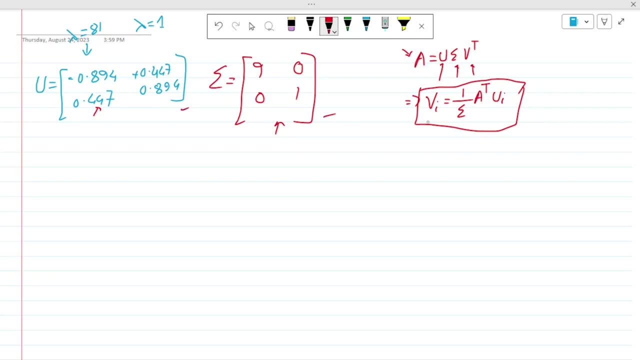 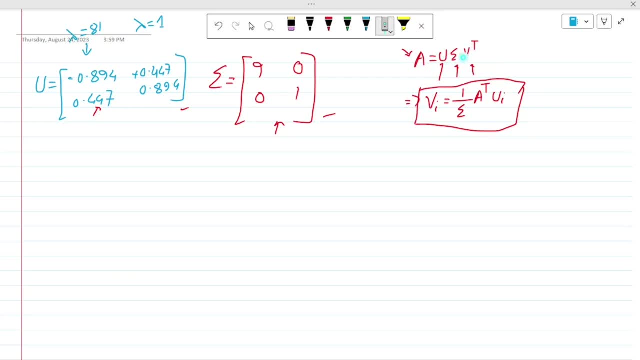 one. so from vt this sigma will come this side, right, so we are finding out v equal to. so v equal to means sigma will come this side. so it is 1 by sigma. then u also will come this side and a because it is transpose. so we are finding our normal v. that means the entire thing will be transpose. 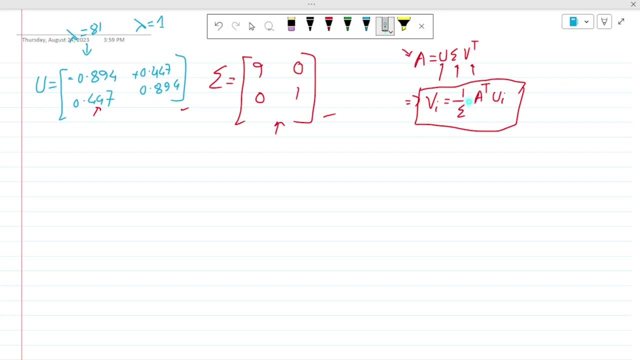 a will be transpose now. so this is the matrix. if we solve it, we will find it out the v matrix. so let's find it out v matrix now. so now here we have a two sigma value, right sigma one, and sigma value. lambda value is 1 and lambda value is 81. so let's do it now. so first case is when 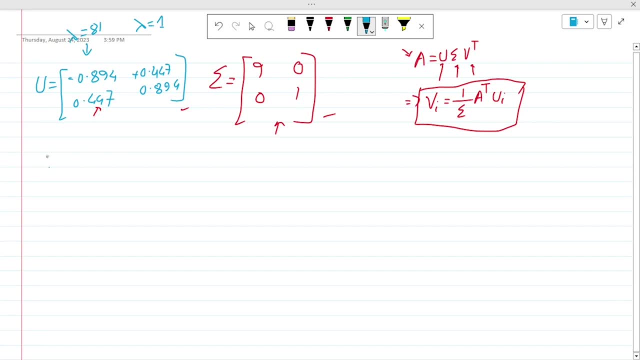 sigma equal to. let's take another color, so sigma equal to. let's take green, so sigma is equal to. let's consider 81. so when sigma is 81 here, so what will be the v? so here again, v12 and v 1: 1, v 1: 1 and v 2: 1. so this value, we have to find it out. so this will be 1 by lambda, 1 by. 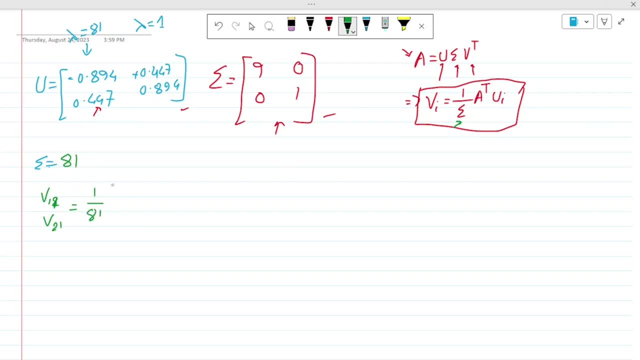 sigma. so sigma value is 1 by 81, 1 by 81 into a transpose, so a, a matrix. if you recall, we had original a matrix in this form, so a matrix. in the equation it is given minus 4, minus 7 and 1. 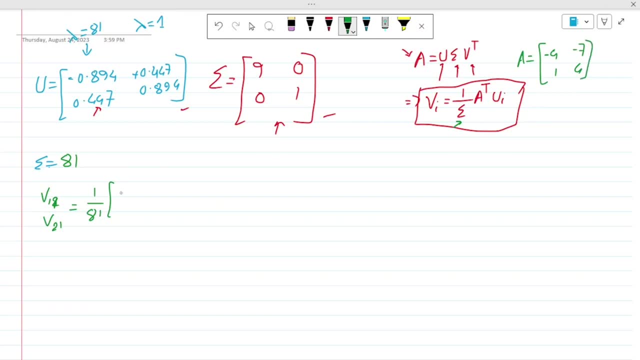 and 4. so what was a transpose then? a transpose will be minus four, minus seven, one and four. so this is our a transpose, a transpose, and you, I, you even sweat first eigen vector. so for for lambda is equal to 81 UI. is this two value? so you? 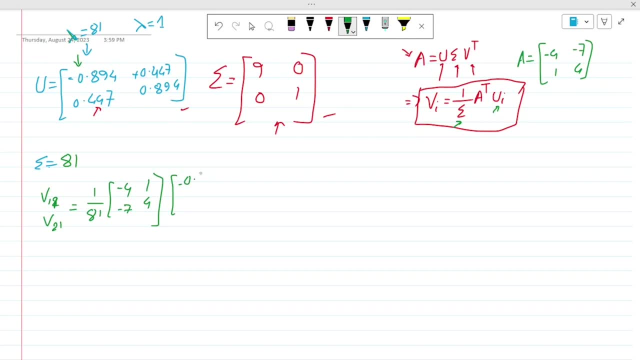 I is this one minus zero point eight, nine four and the zero point four four seven, because here Sigma value we used 81, right, so Sigma will we use it. even means: here we put Sigma value, we used 81, right so Sigma value, we used 81. means here we put Sigma value, we use 81, right so Sigma value, we. 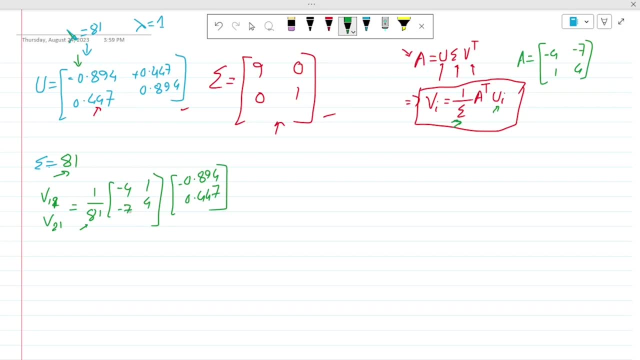 81, 81 and a transpose. is this one and a transpose into ui. ui means what eigenvector when the sigma was 81, so eigenvector for sigma 1 sigma was 81. is this value? so this was the sigma value when 81 we calculated eigenvalue. is this one so the same value? we have written it here. now, if we 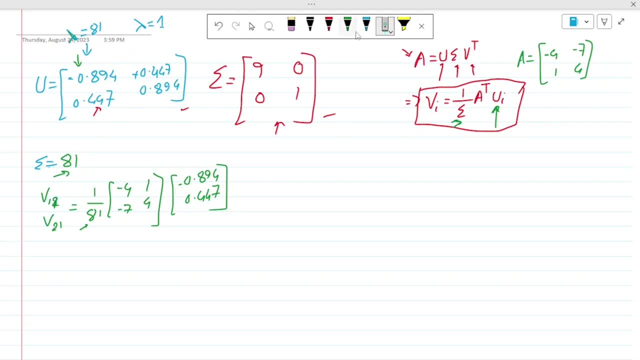 multiply all these three, you will get v 1- 1 and v 1, 2. so let's do it here very simple. so it is again matrix multiplication. so once you do this matrix multiplication, the final value you get it is 0 point 4, 4, 7 and 0 point 8, 9, 4. so this is the matrix multiplication. ok, let me just do it one. 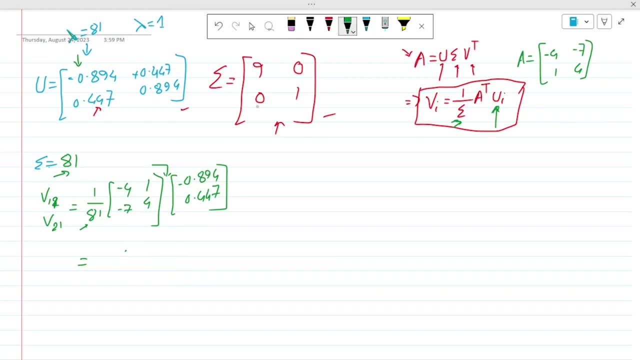 line for you, then you can do the remaining part. so let me do it one line. so 1 by 81, then I am multiplying by 1 and I am multiplying by 1, and I am multiplying by 1 and I am multiplying by 1. 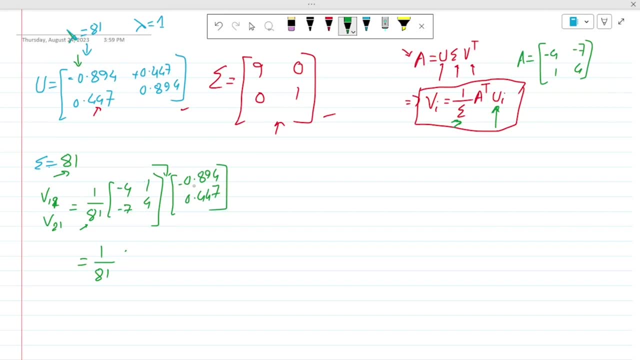 this matrix with this matrix. so minus 4 into minus this value. so the first value will be minus 4. into minus 0 point 8, 9, 4 right and 1 plus, so it will be plus. so this is one value, entire value, plus 1 into this value. so 1 into this value is 0 point 4, 4, 7. similarly, at the 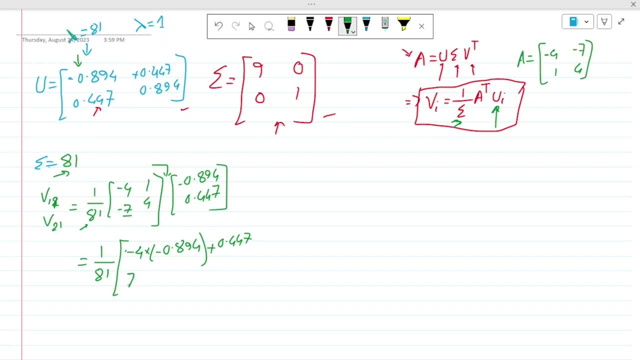 bottom. it will be minus 7 into this one, so minus 1 is plus. so it will be 7 into 0 point 8, 9, 4, plus matrix multiplication plus 4 into this value. so plus 4 into 0, point 4, 4, 7. so this is the. 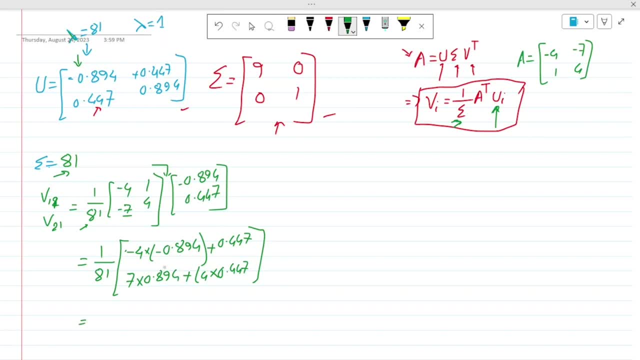 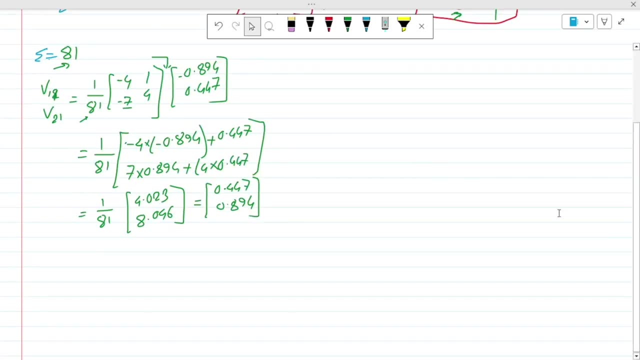 matrix. you will get it so and you compute this value and bottom value and you divide it by 81 for both the values and then simplified value. you will get it. so if you simplify the values. you will get it. so if you simplify the values. you will get it. so if you. 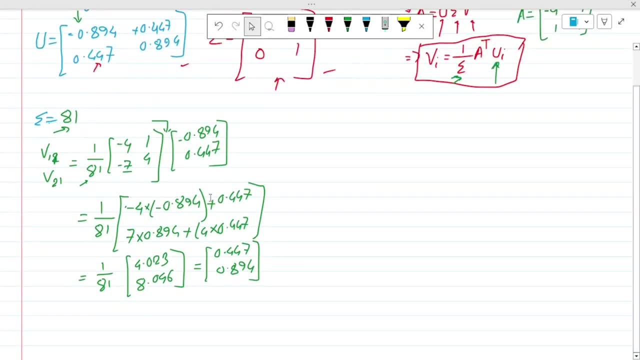 simplify this equation, you will get it. if you solve this equation, you will get it: 4.023 and 8.046 and this, this lambda value, is actually root, square root of 81. just, we just make a correction. this is square root because lambda value, we got it 81. so sigma value will be square root of 81. 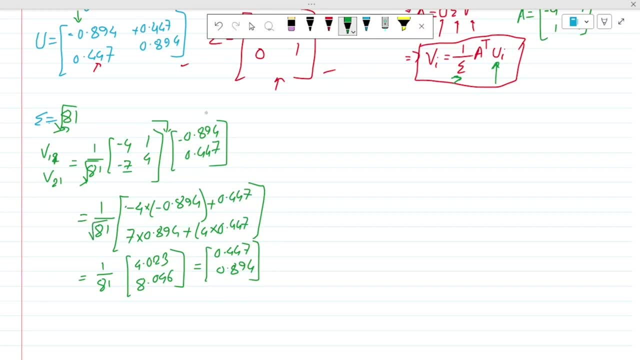 so this will be always square root of 81. so square root of 81 means nothing but a 9. so this value will be 9. so 1 by 9. then if you divide both the values by 9, you will get. so this is the final. 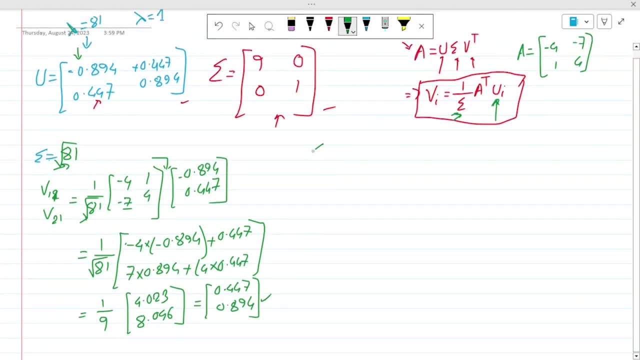 value. so now same thing. we will do it for sigma equal to 1, so sigma is equal to 1. you will get again v 2- 1, sorry, v 1- 2 and v 2- 2, so this two value you will get it same equation, right, so 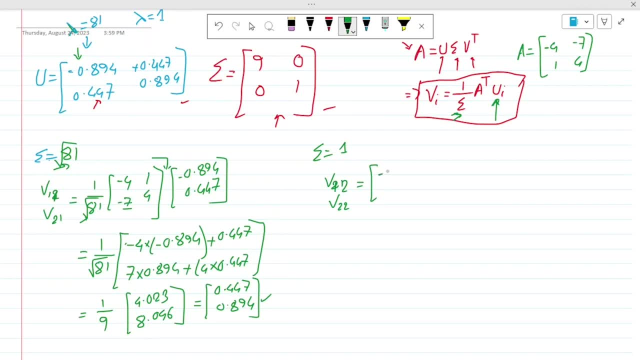 you will get a transpose t, so a transpose is minus 4, 1 minus 7 and 4, so this multiplied by here. now you need vector for 1, so you need vector. so eigenvector for lambda is equal to 1, is this one? so this multiplied by this one, so 0.447. 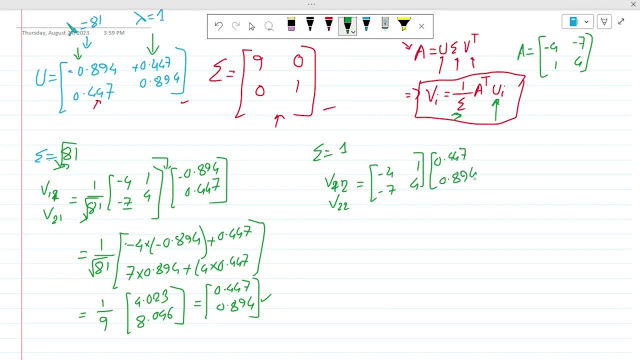 by 0.894. so these are the two matrices. again it is matrix multiplication. so here sigma value is 1, because square root of 1 is 1, so it is 1 by 1. so it is okay. so now we multiply again. you will have minus 4 into 0.447. so this is the first part, then plus 1. 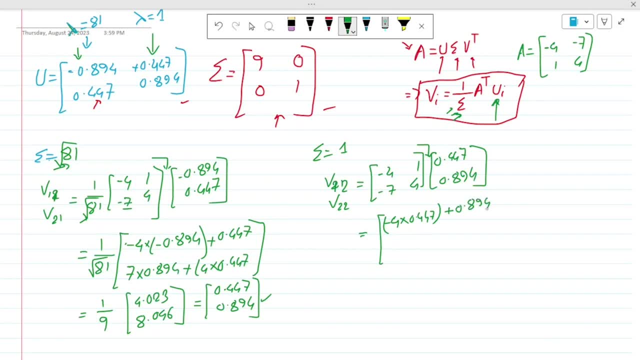 into 0.894. similarly, minus 7 into this value, minus 7 into 0.444, 4 for 7 plus 4 into 0.894. so now, if you simplify this, you will get the simplificates simplified equation of simplified vector of minus 0 p гол 2 plus 0 p 0.. if you simplify this, you will get the simplified equation of simplified vector of minus 0.99. 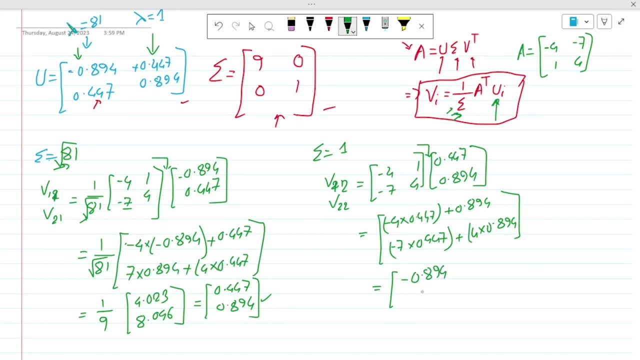 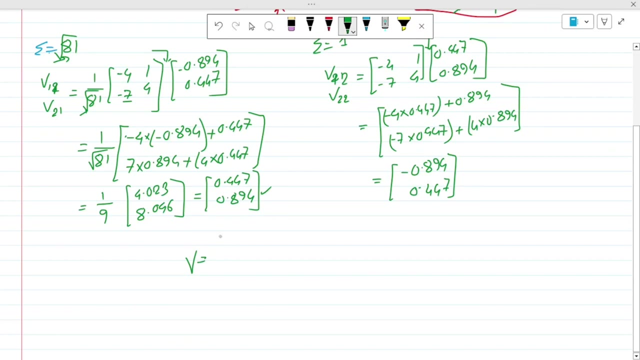 0.894 and here you will get 0.447. so now final V matrix. we got it now. if you combine both, you will get the final V matrix. so final V matrix is this two value, which is 0.447 and 0.894, and from here you will get minus 0.894 and 0.447. so this is our third V matrix. so now,